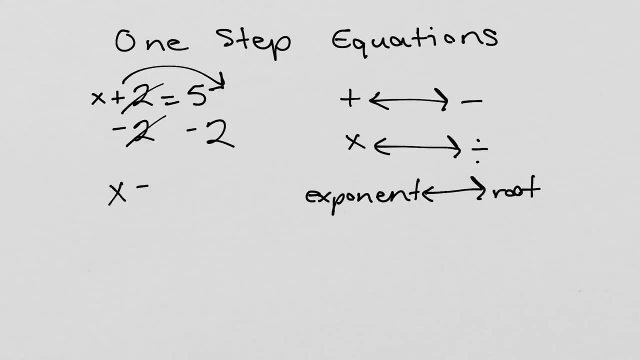 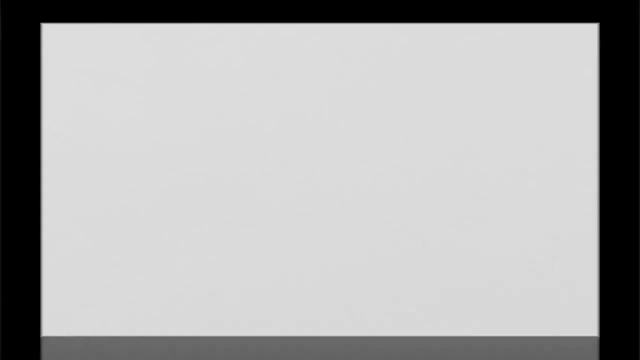 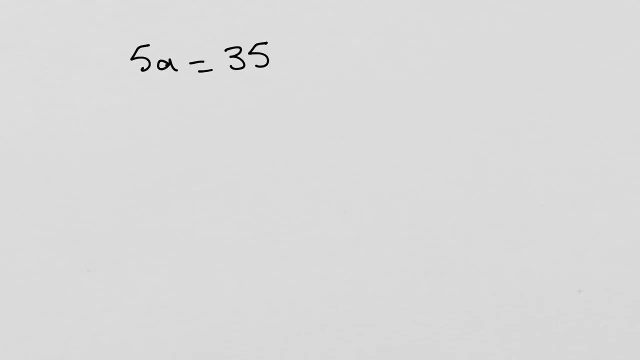 Solve for a. Solve for a. Here again, we want to get rid of anything that is with the a. This means we have to get rid of the 5.. So 5a is the same as 5 times a. Since the 5 is multiplying, we will perform the opposite operation on it. 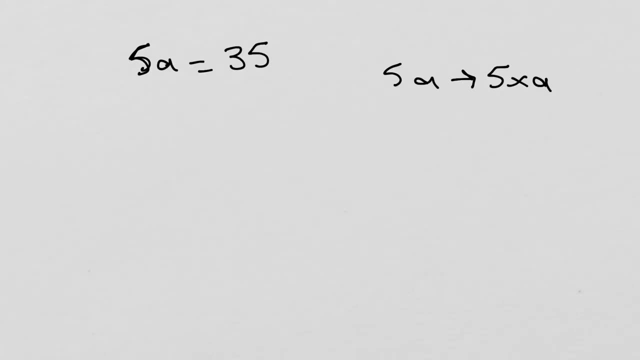 We know that the opposite operation of multiplication is division, so we will divide both sides by 5.. Since we performed the opposite operation, we can say that the 5 will cancel out. Now, 35 divided by 5 is 7.. So a equals 7.. 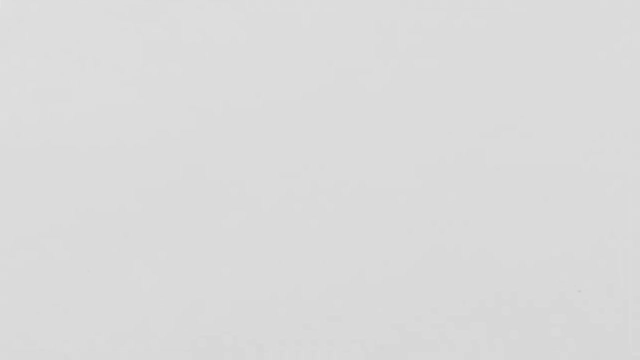 Now try these questions and leave your answers in the comments section. Number 1,: solve for x and x over 9 equals 3.. Number 2. Solve for x and x minus 6 equals 12.. Number 3,: solve for b and 3b equals 18.. 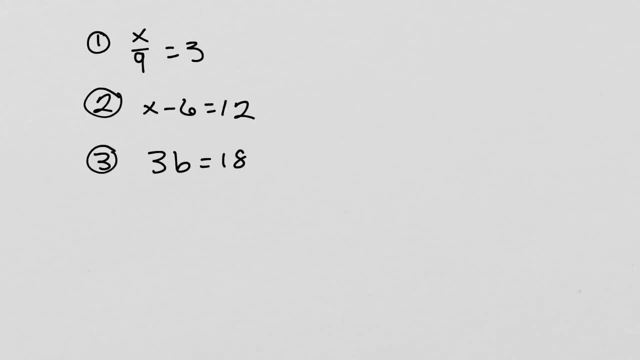 Remember, you are just performing the opposite operation on both sides. So in the first question, for example, the 9 is dividing. We will perform the opposite operation on both sides. So in the first question, for example, the 9 is dividing. 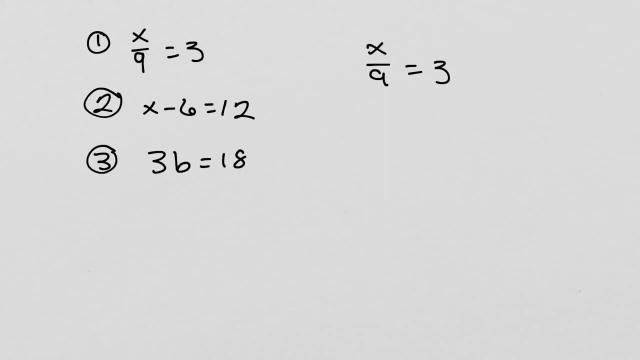 We will perform the opposite operation on both sides of the equation, so you will have to multiply both sides by 9.. The 9 will cancel out, since we performed the opposite operation on it 3 times. 9 is 27,, so x will be 27.. 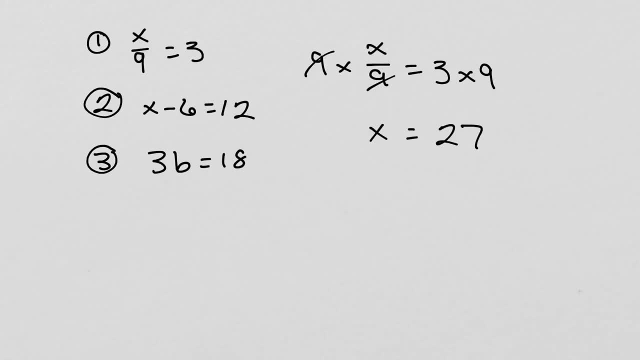 Okay, I'll leave the next two for you. In the examples we've done so far, we needed to perform only one operation to solve the questions. So for our first example, we just did subtraction. For our second example, we just did division. 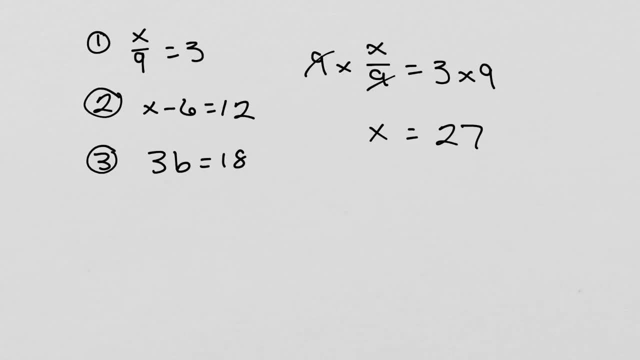 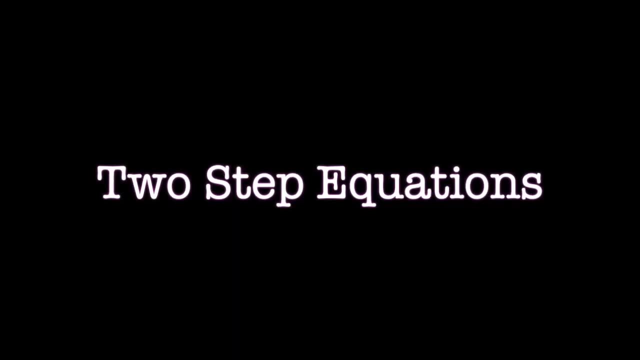 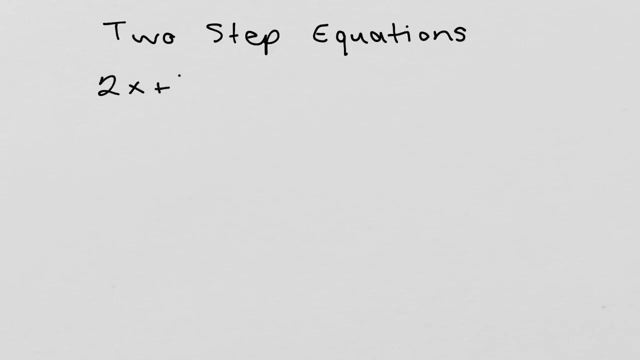 And for this one we just did multiplication. That is why they are called one-step equations. Two-step equations. Let's look at an example to explain it. 2x, 2x plus 3 equals 11.. Solve for x. 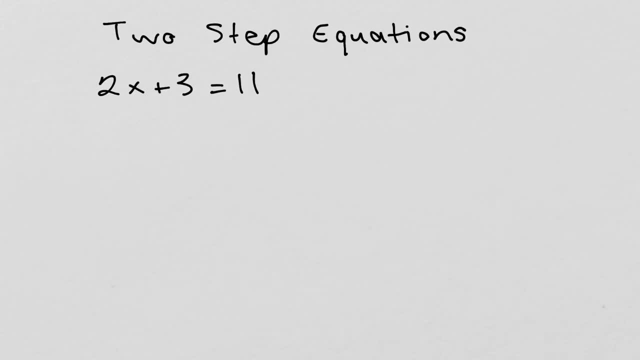 We said earlier that the whole idea of solving equations is to get rid of everything and leave the x on one side of the equation. For this question, we will see that we have to get rid of the multiplication by 2 and the plus 3.. 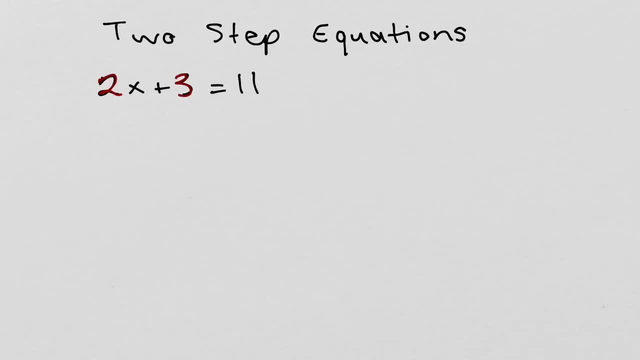 Remember we said 2x is the same as 2 times x. When there are more than one operation, we use the idea of the reversal. So here is the reversal of the order of operations to know which one to get rid of first. 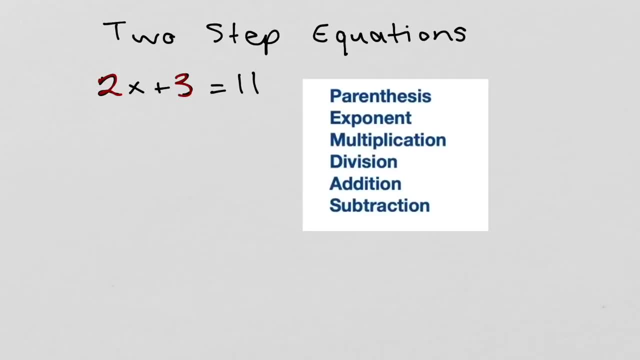 So here is the order of operation. If you are not familiar with the order of operation, we've put a link in the description for you to master it. It's important that you watch it. Knowing the order of operation will make solving of equations super easy. 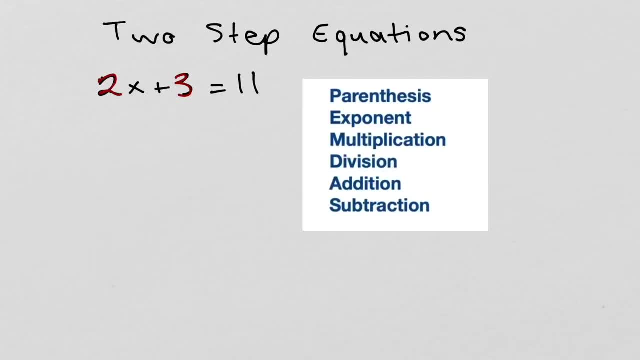 We can see that in the reversal of the order of operation we have addition first and multiplication second, So we will get rid of the plus 3.. We get rid of the plus 3 by performing the opposite operation on it, So we will subtract 3 from both sides. 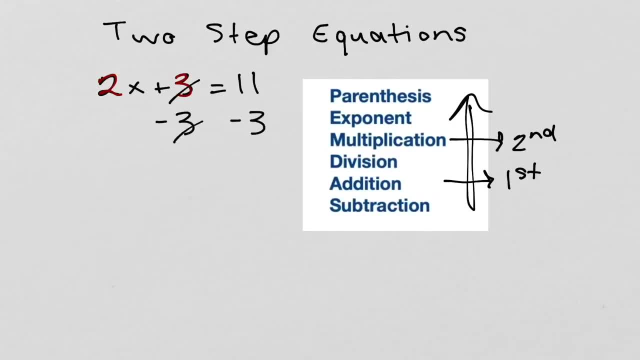 The 3 will cancel out. 11 minus 3 is 8.. So we have 2x equals 8.. Next, we will get rid of the plus 3.. Next, we will get rid of the plus 3.. Next, we will get rid of the plus 3.. 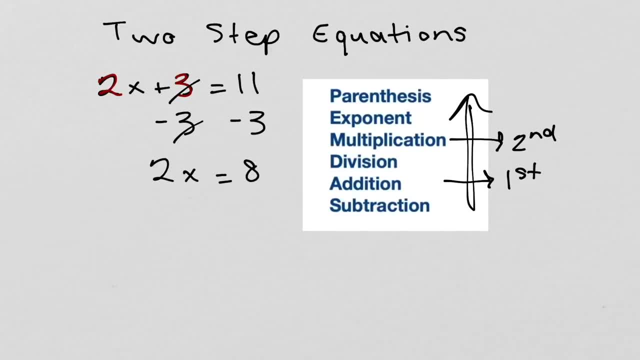 We will get rid of the multiplication by dividing both sides by 2, since division is the opposite of multiplication, The 2 will cancel out. 8 divided by 2 is 4.. Therefore, x equals 4.. Before we take more examples, 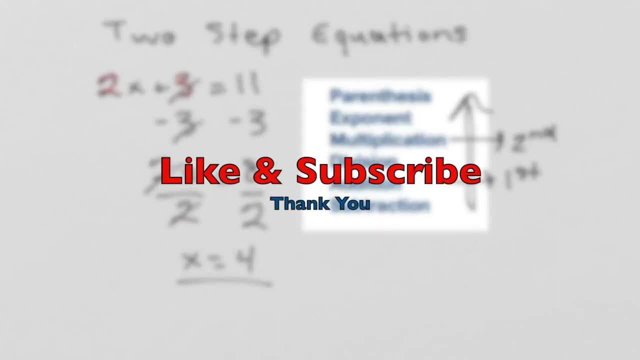 we want you to do us a huge favor by liking this video. This is really the best thing you can do to encourage us to make more videos. This is really the best thing you can do to encourage us to make more videos. If we don't know, you like the videos. 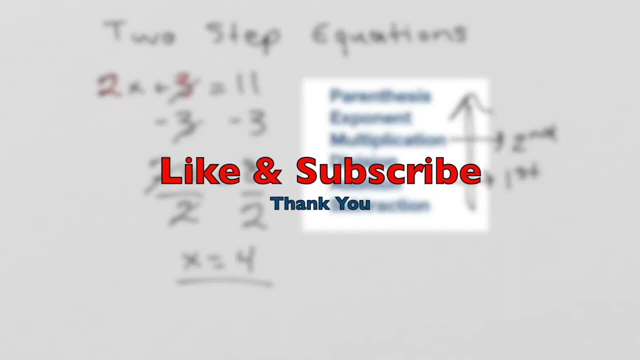 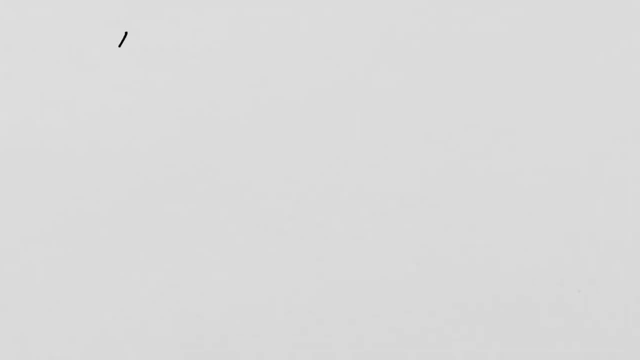 we won't have any reason to post more. Okay, let's take our next example. Solve for x and x over 3 minus 4 equals 6.. We want to get rid of all the numbers attached to the x so we can have the x alone on one side of the equation. 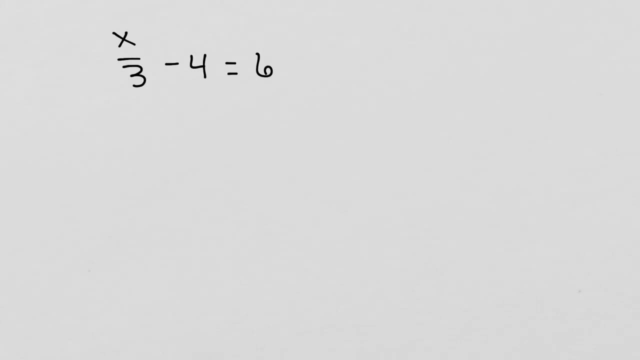 To achieve this, we know that we must get rid of the divided by 3 and the minus 4.. Let's write our order of operation, Please. you don't need to be writing the order of operations in your solutions. at school, We are using it for teaching purposes. 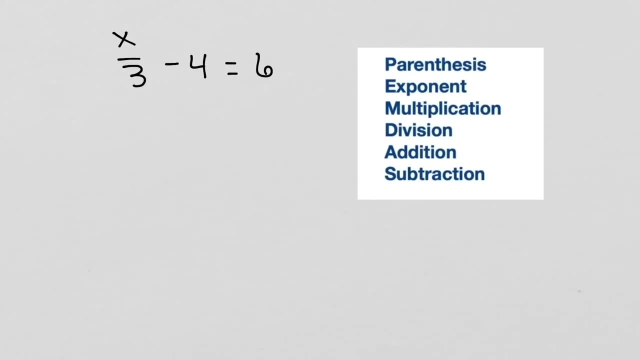 We are using a reversal of the order of operations, so we are working from the bottom up. We will see that in this form we must do subtraction first, division second and division second To get rid of the minus 4, we must perform the opposite operation. 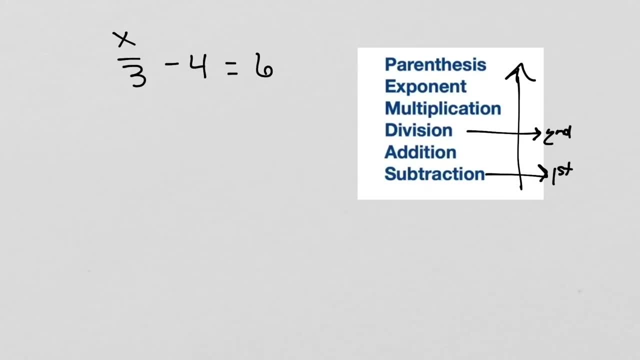 on both sides of the equation. So we will add 4 to both sides. The 4 will cancel out. 6 plus 4 is 10.. We now have x divided by 3 equals 10.. Next we will get rid of the divided by 3.. 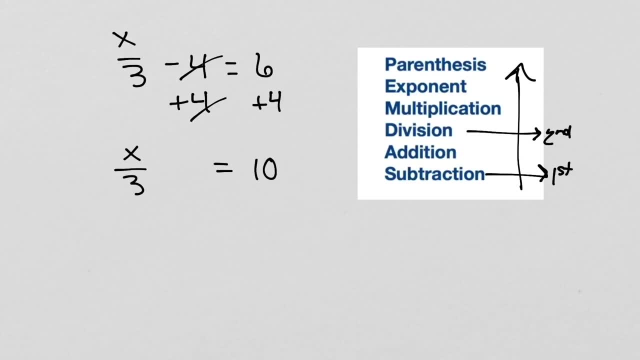 We do this by performing the opposite operation on both sides of the equation. So we will multiply both sides by 3.. The 3 will cancel out. 10 times 3 is 30. Therefore x equals 30.. In most instances for two-step equations, 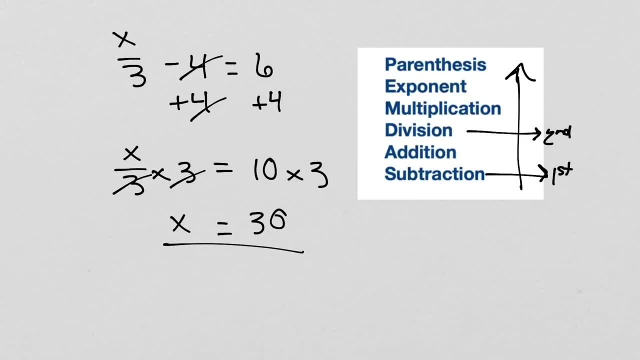 you will work out your addition or subtraction part first. Then you will work out your multiplication or division part next. Please, this is not always the case. Topics like this requires practice, practice, practice. You want to be so good at it that you don't need to use 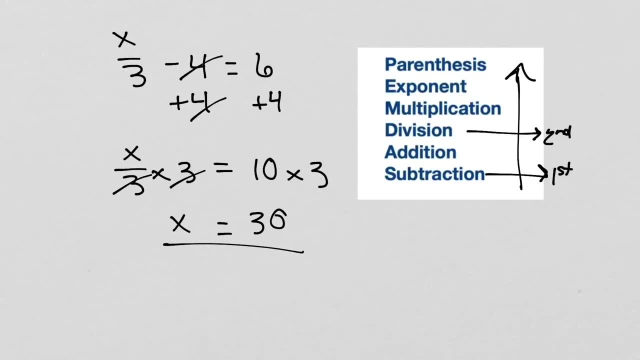 the reversal of the order of operations anymore. You see a question and you just know which one to do first and second. You can get more practice with the link in the description. Try the following and leave your answers in the comments section, Number 4.. 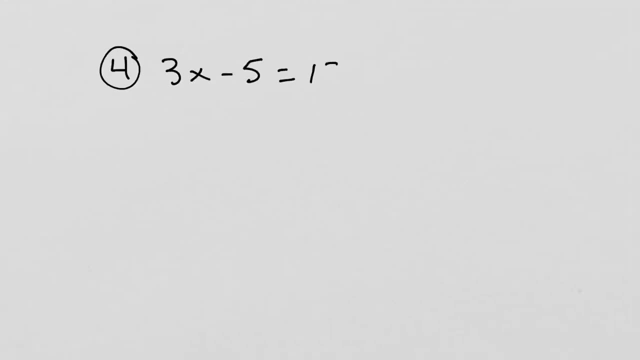 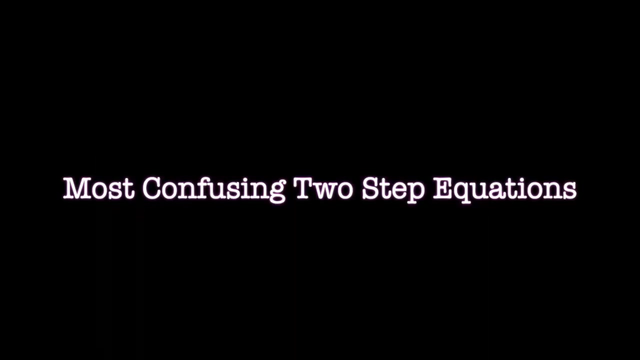 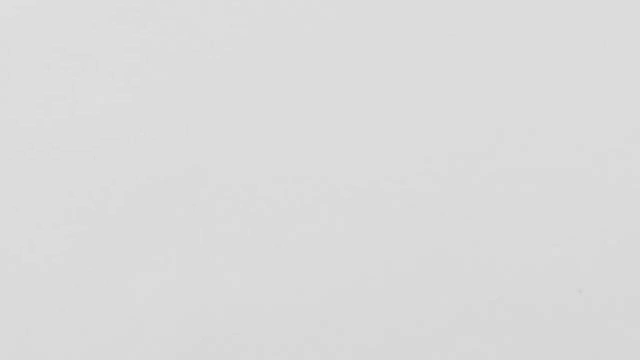 3x minus 5 equals 13.. Solve for x Number 5.. x over 5 plus 3 equals 8.. Solve for x. Most confusing two-step equations: Two-step equations that require distribution or has an operation in parentheses is the. 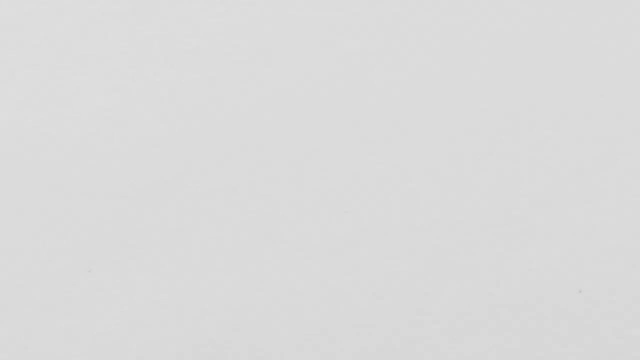 one most students get confused with. In fact, not all math teachers agree that this is a proper two-step equation, but it is. Let's look at 2 parentheses: x plus 5 equals 16.. We will solve it two ways. Method 1.. 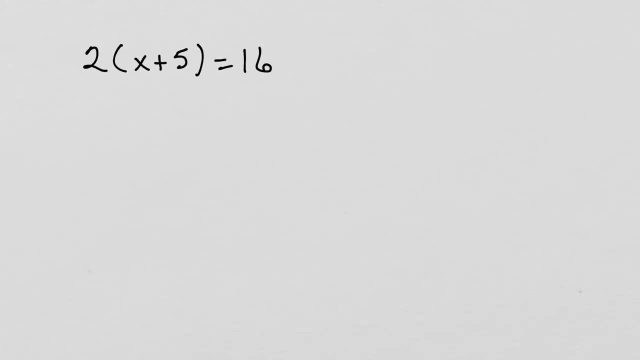 We will first distribute the 2.. The 2 will multiply everything in the parentheses. So the 2 will multiply the x to get 2x, plus the 2 will multiply the 5 to get 10.. We have: 2x plus 10 equals 16.. 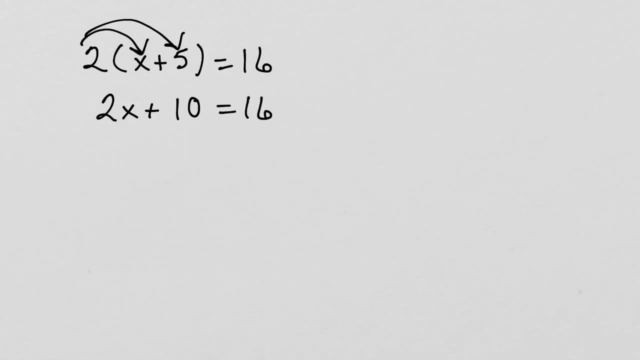 We can see that we have a familiar two-step equation. Let's write our order of operation AT: x is equal to x, to the x to the y and u equals 5.. The time period to know which is our number of Milwaukee roots can't be altered. 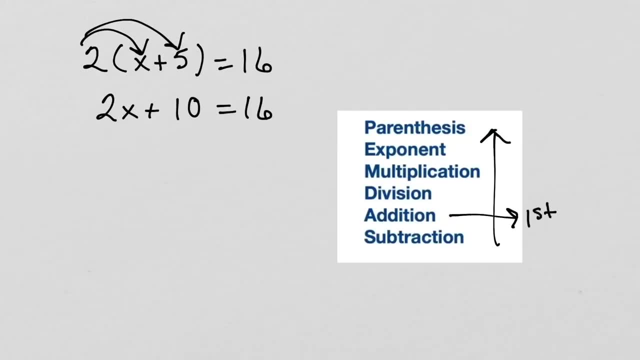 By using the reversal of the order of operation. we will do the plus 10 first And then the times 2. 10. by subtracting 10 from both sides, the 10 will cancel out. 16 minus 10 is 6. so 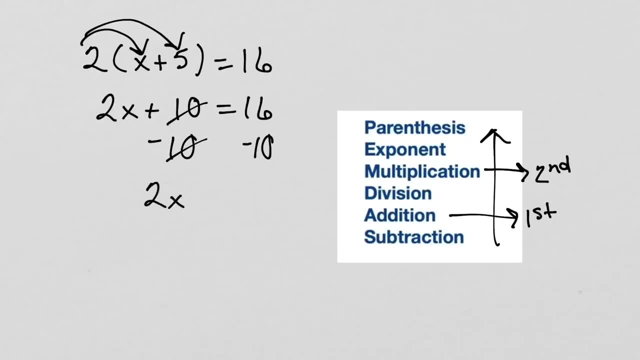 we have: 2x equals 6. next we will get rid of the times 2 by dividing both sides by 2. the two will cancel out. 6 divided by 2 is 3, so X equals 3. here you realize that we did an extra step of distribution. 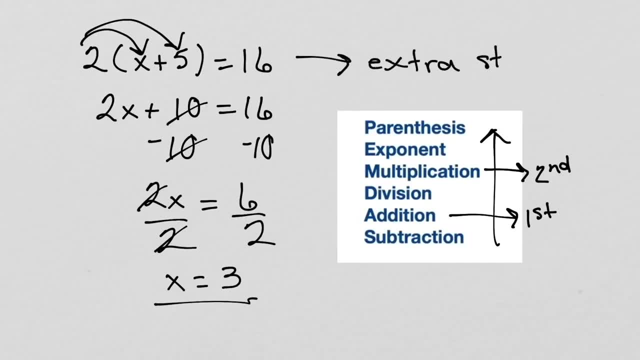 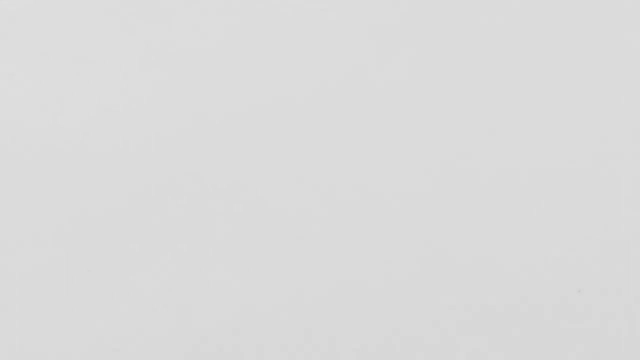 before we could apply the two-step equation. you can solve it this way if it's easy for you, but that's not the best way to solve it. let's look at method 2 for the purpose of teaching. we're going to break this down, but your goal is to be familiar with questions. 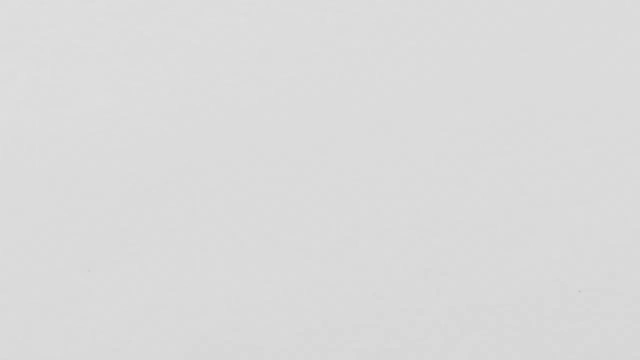 like this, so that you don't need all this breaking down and thinking to solve it. let's write the question down and we're going to write the answer down and we're going to write the order of operation again. in the order of operation, parentheses are performed first. 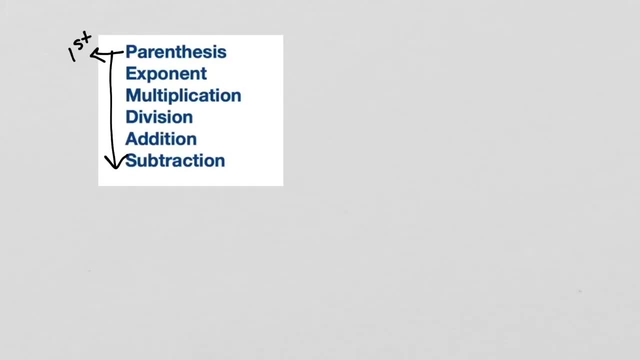 when we say parentheses are performed first, what we actually mean is that the operation of parentheses is performed first. so if we have 2 times parentheses- 2 plus 4- then we will perform the 2 plus 4 first because it's in parentheses. so basically, we perform the addition operation first because it's in parentheses. 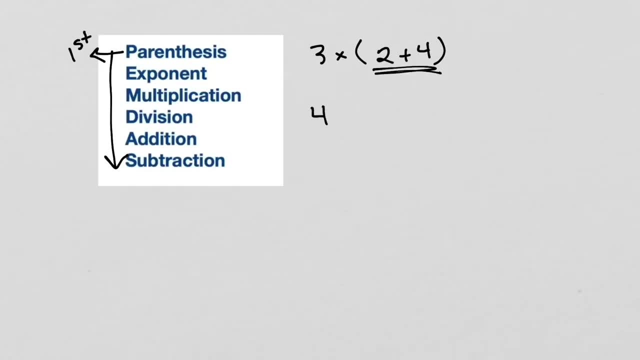 similarly, if we have 4 plus 6 parentheses, 2 times 7, exponent 3, we will perform the 2 times 7 first because it's in parentheses. so we perform the multiplication operation first because it is in parentheses. now, since we know that equations are solved with the reversal of the order of 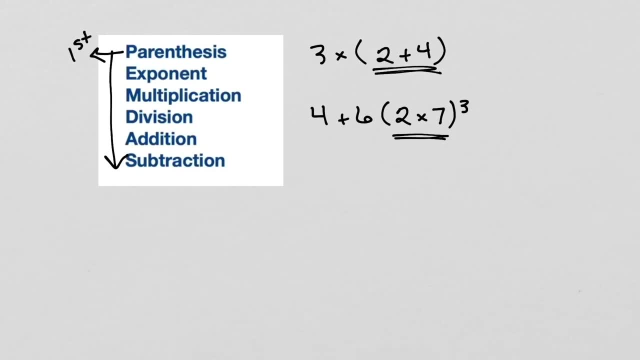 operation. it means that we will solve the operation in the parentheses last. with that in mind, let's look at our question. 2 parentheses x plus 5 equals 16. remember: 2 parentheses x plus 5 equals 16. x plus 5 is the same as 2 times parentheses x plus 5.. Here, since the x 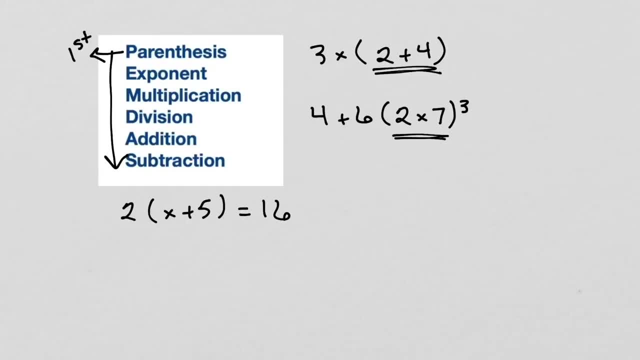 plus 5 is in parentheses. we will call it a parentheses operation. So we have multiplication operation and a parentheses operation. Using the reversal of the order of operation, we will do the multiplication first and parentheses last. We get rid of the times two by dividing both sides by two. 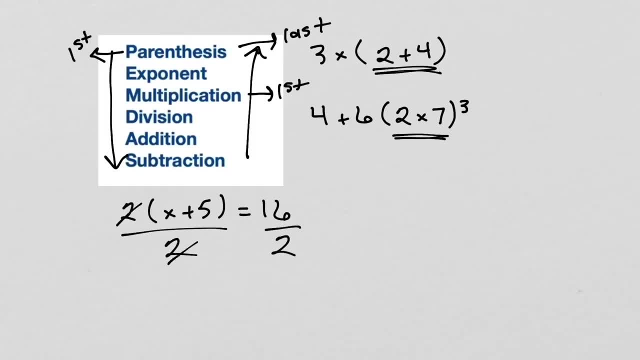 The 2 will cancel out. 16 divided by 2 is 8.. Now we can remove the parentheses to get: x plus 5 equals 8.. Once you're about to perform the operation in parentheses, you can remove the parentheses. We will get rid of the. 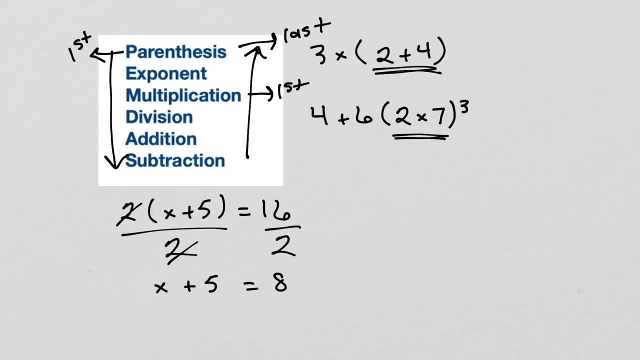 plus 5. by subtracting 5 from both sides, The 5 will cancel out. 8 minus 5 is 3, therefore x equals 3.. You will realize that here we did only two steps. therefore, this is a true two-step equation. 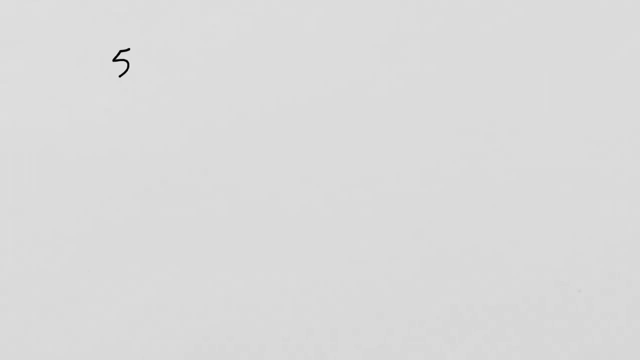 Try this question. Five parentheses: x minus 7 equals 55. solve for x. Pause the video and try it first. We can see that we have a multiplication operation and an operation in parentheses. Using the reversal of the order of operation, we will do the multiplication operation and the operation in parentheses. Using the reversal of the order of operations, we will do the multiplication. 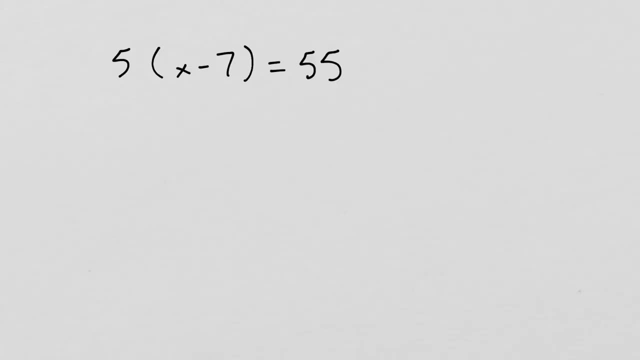 operation first and then the operation in parentheses. We remove the times 5 by dividing both sides by 5.. The 5 will cancel out. 55 divided by 5 is 11.. So now we have: x minus 7 equals 11.. 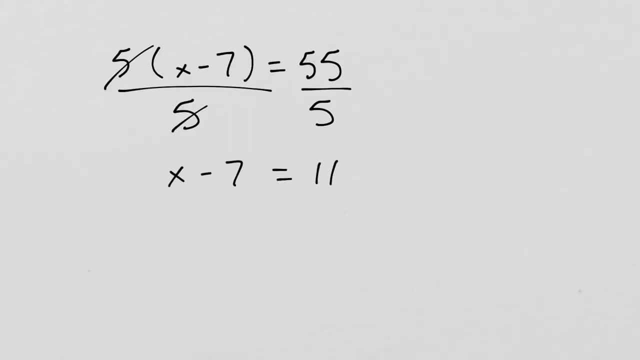 Again, once you're about to perform the operation in parentheses, you can remove the parentheses To remove the negative 7, we will add 7 to both sides of the equation. The 7 will cancel out. 11 plus 7 is 18.. So x equals 18.. 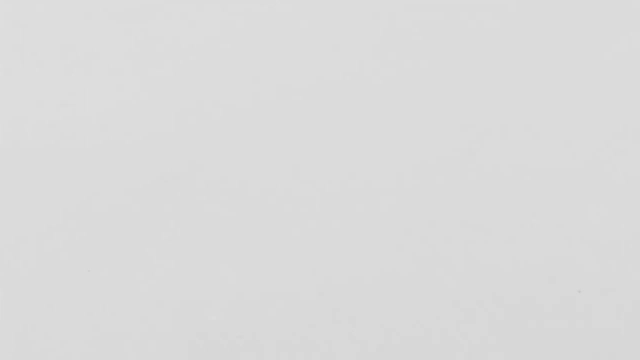 Let's look at parentheses: x minus 6 over 4 equals 6.. Please pause this video and try it before you watch our solution. Here we have a division operation and an operation in parentheses. Let's write our order of operation From the reversal of the order of operation. we have to do division first. 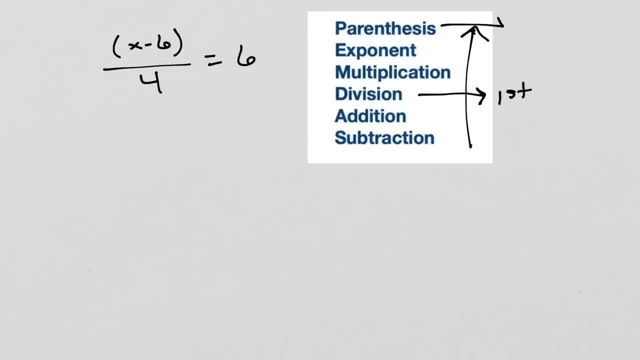 and parentheses. last, We get rid of the divided by 4 by multiplying both sides by 4.. The 4 will cancel out. 6 times 4 is 24.. Now we can remove the parentheses to have x minus 6 equals 24.. 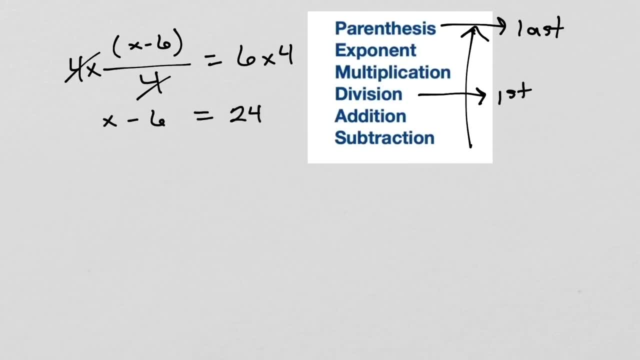 We get rid of the minus 6 by adding 6 to both sides. The 6 will cancel out. 24 plus 6 is 30. Therefore, x equals 30.. When it comes to division, the parentheses is usually not written, So parentheses x. 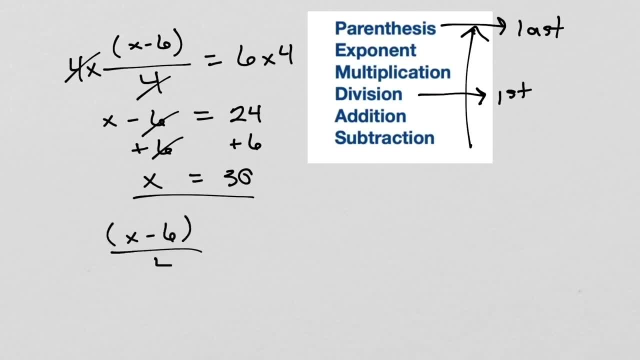 minus 6 over 4 will be simply written as x minus 6 all over 4.. When you say number dividing two or more numbers, this way parenthesis is implied. A plus B plus C all over 5 is the same as parentheses A plus B plus C all over 5.. 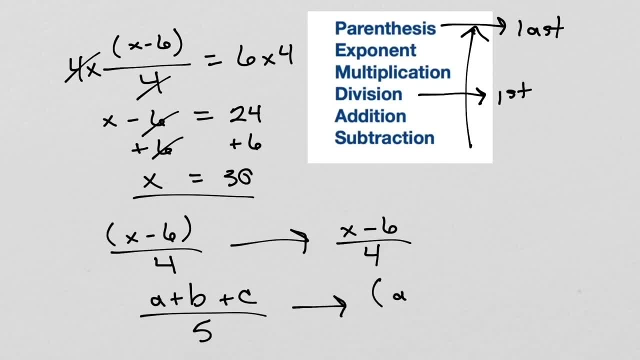 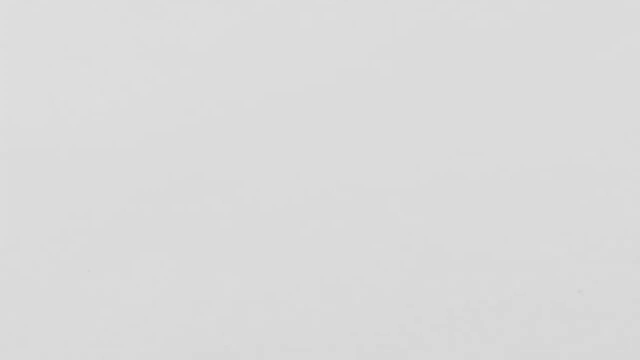 It will be the same if we do a new division operation. The gate is now open. So if we have said the number division, the number division operation is the same for the addition of the numbers, right? please try these and leave your answers in the comments section, number 6: 3. 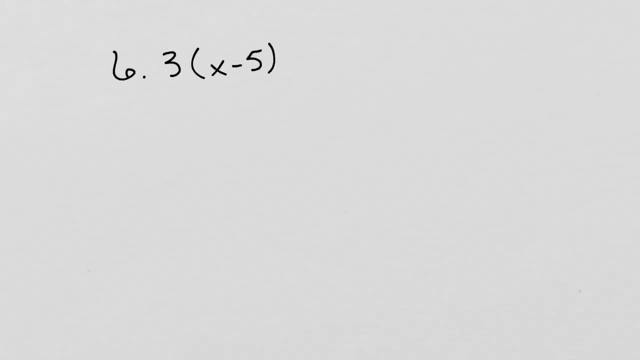 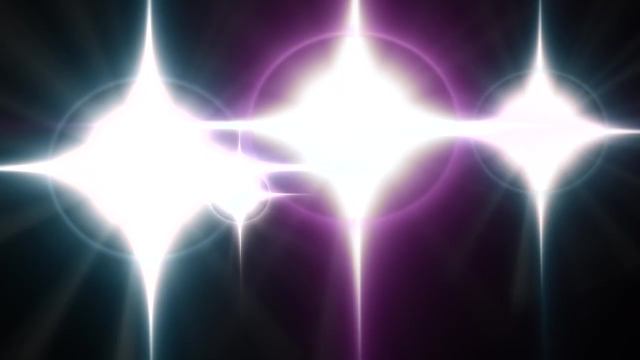 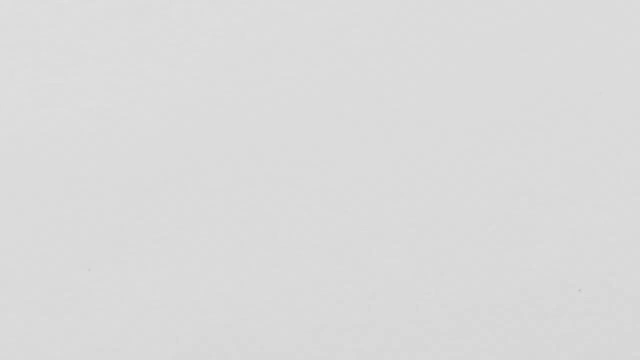 parentheses: X minus 5 equals 21. number 7: X plus 4. all over 7 equals 6. multi-step equations is used to imply any equation that you need to perform more than one operation in order to solve it, so two-step equations is actually an example of multi-step equation. let's use this example to: 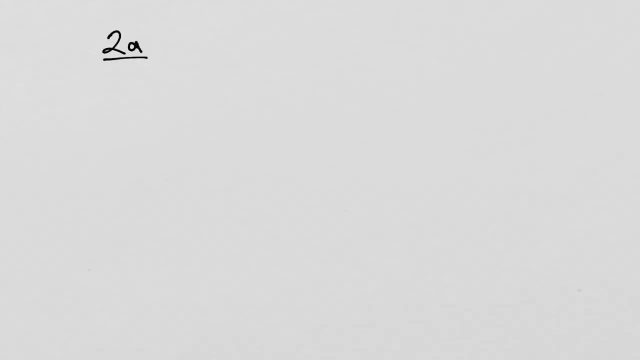 explain it: 2a over 7 minus 5 equals 3. solve for a. the process of solving here, as c is the divisible matrix, add the包 macrame by www dot cdip length minus three up we divide around. that the matrix is Solving is nothing different from what we did to solve two-step equations. 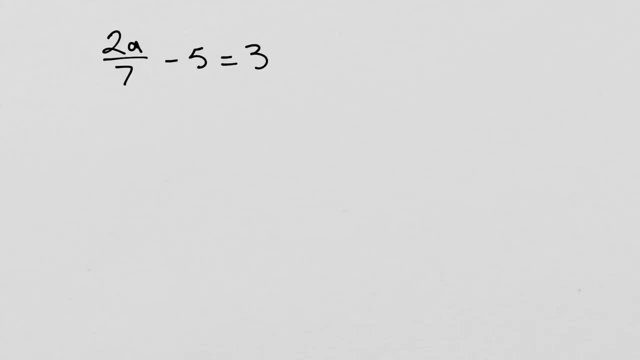 We want to get the a on one side of the equation, So we have to remove the times 2, the minus 5, and the divided by 7.. We remove them by performing the opposite operation on them. We know that the opposite operation of addition is subtraction. 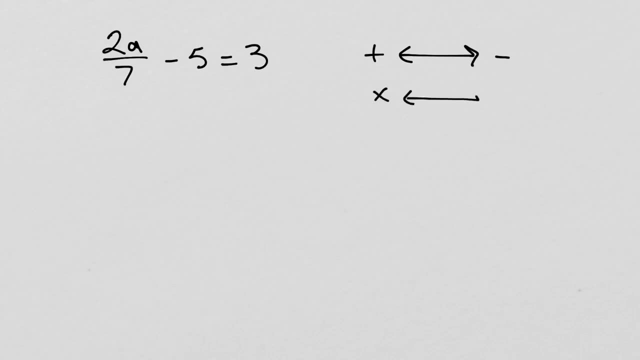 The opposite operation of multiplication is division And the opposite operation of exponent is roots. We also know that in order to know which operation to perform first, we will use the reversal of the order of operation. So here is our order of operation. So, using the reversal of the order of operation, we will see that we have to do the minus 5. 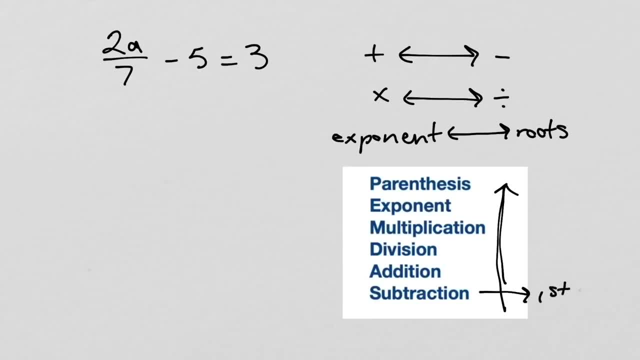 first, then we will do the division by 7, next and finally the times 2.. We get rid of the minus 5 by performing the opposite operation on it, So we'll add 5 to both sides. The 5 will cancel out. 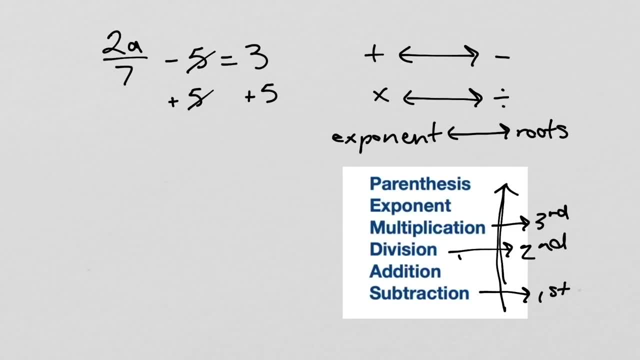 3 plus 5 is 8.. So now we have 2a over 7 equals 8.. We know we will do our division. next We get rid of the divided by 7 by performing the opposite operation on it, So we will add 5 to both sides. 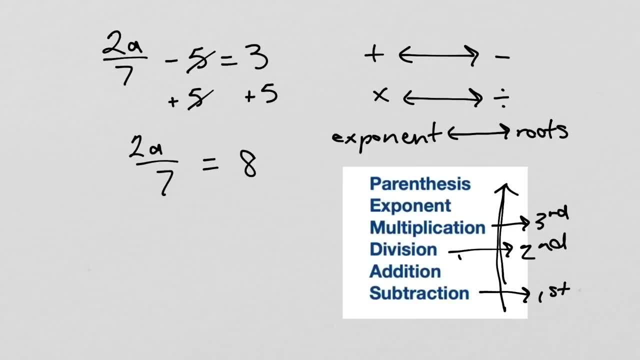 The 5 will cancel out the opposite operation on it. We will multiply both sides by 7.. The 7 will cancel out. 8 times 7 is 56, so now we have 2a equals 56. Finally, we will get. 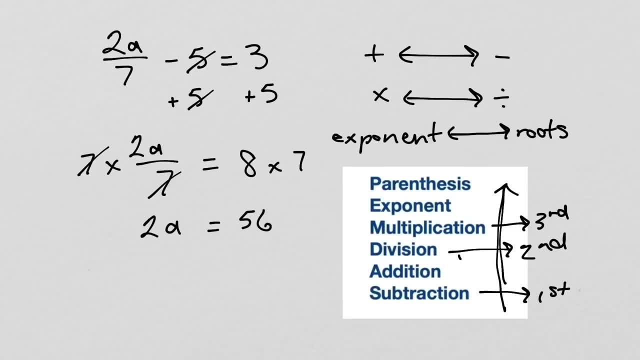 rid of the times 2 by performing the opposite operation on it. So we'll divide both sides by 2.. The 2 will cancel out. 56 divided by 2 is 28,, therefore a equals 28.. So here you can see that it's really just like the two-step equation We are. 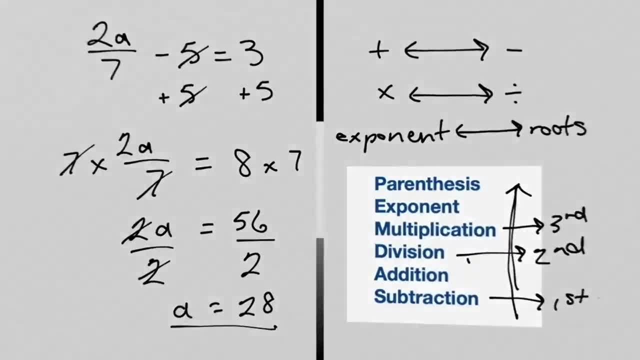 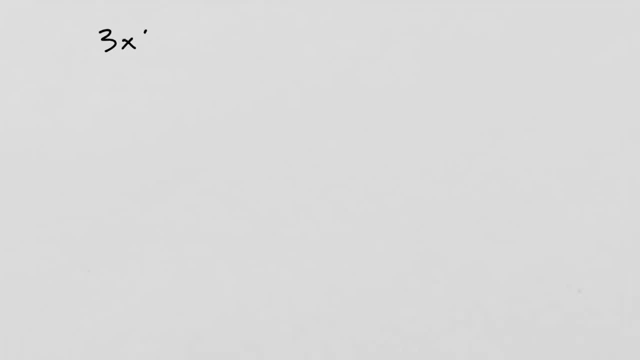 just doing more steps. Let's take another example: 3x squared plus 8 equals 20.. Solve for x. Here again, we want to get the x on one side of the equation. In order to do that, we have to. 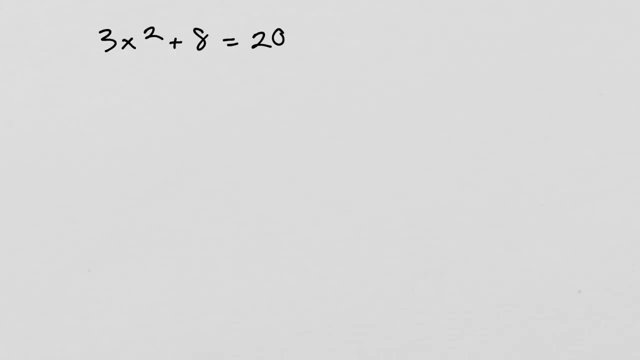 get rid of the multiplication by 3, the exponent 2, and the plus 8.. We will use the reversal of the order of operation to know which one to perform first. Let's bring our order of operation. So here is our order of operation. In the reversal we will notice that we have to do: 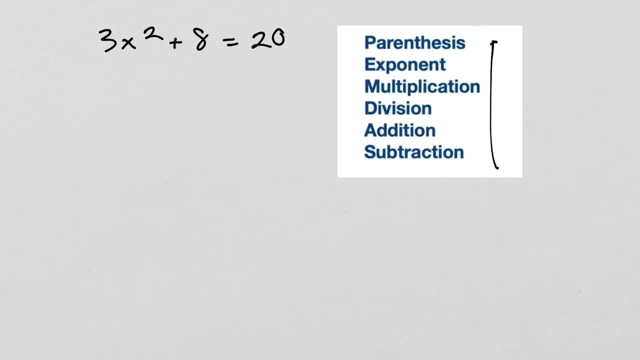 the plus 8 first, Then we will do the multiplication by 3. And then we will do the exponent 2.. We will get rid of the plus 8 by performing the opposite operation on it: Subtract 8 from both sides. The 8 will cancel out. 20 minus 8 is 12.. So now we have 3 times 2. So it's greater. than increasing 7.. Ok, so now we know which two- غ선 is different. Now we need to write bgc, because bgc is sen of P От. So now we need to write: bgc equals how many times 2 a is equal to 6.. 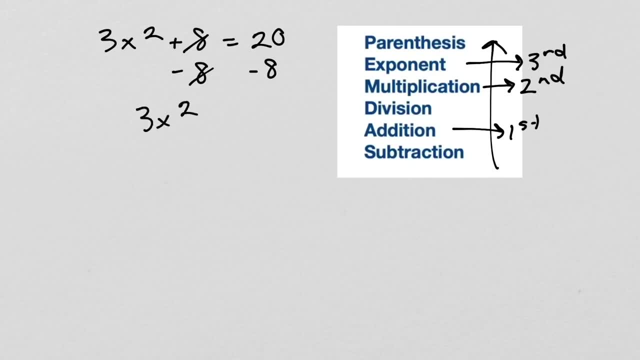 So now we get rid of the plus 8 by performing the opposite operation on it. I will derive the plus 8 by performing the opposite operation on it. Subtract 8 from both sides, x squared, equals 12.. Next we have to get rid of the multiplication by 3. We do the 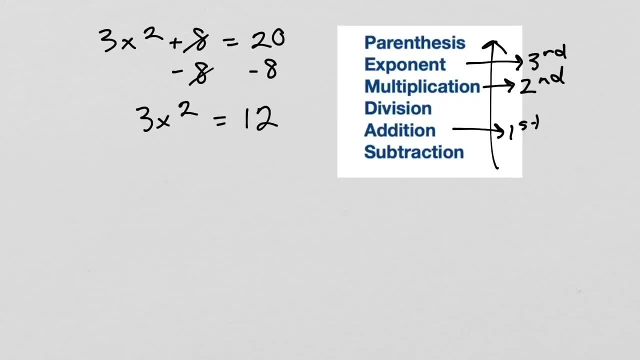 opposite operation. We divide both sides by 3.. The 3 will cancel out. 12 divided by 3 is 4.. So now we have x squared equals 4.. We finally have to get rid of the exponent 2.. We do the opposite operation. The opposite operation of exponent 2 is square root. We. 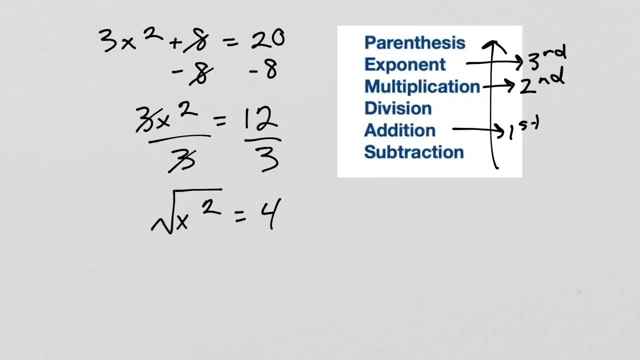 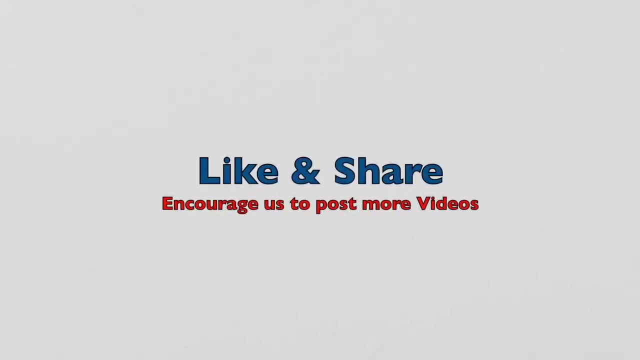 find the square root of both sides. This will cancel out. The square root of 4 is 2.. Therefore, x equals 2.. Hope you are enjoying this video. Please don't forget to like and share this video. It's important you try a lot of questions. Understanding alone is not enough. Practicing will increase. 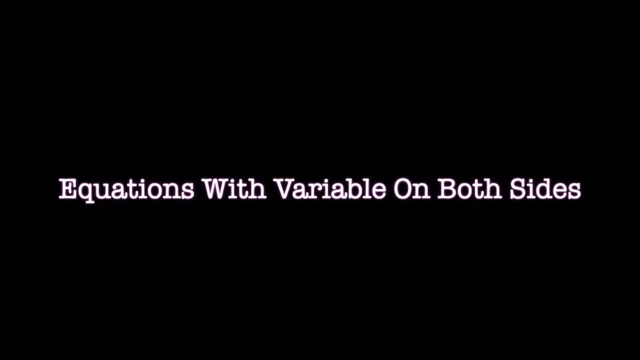 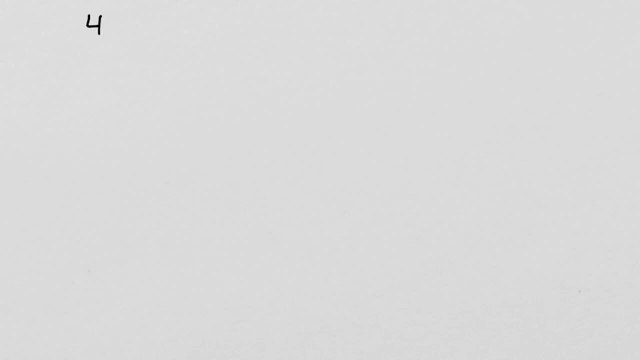 your speed and accuracy. Let's take a question to expand the session. If you want a questions. When compingcuphandion D is 2, When we came from quantum crowding, We need 혹시 to check the problem. explain this: 4x plus 5 equals 9 plus 2x. Solve for x. We have been having the x represented. 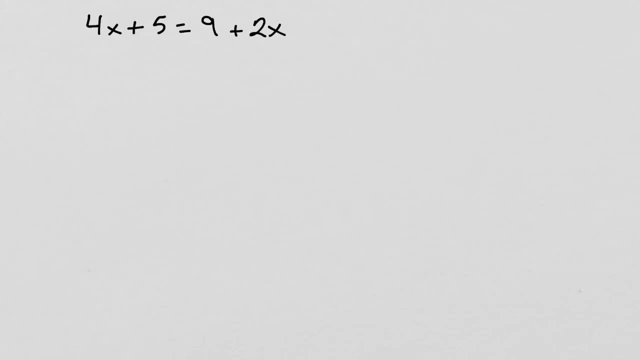 only once. Example: 4x plus 5 equals 9.. But here we have the x represented 2 times. In a case like this, we want to move the x values to one side of the equation and work on it. 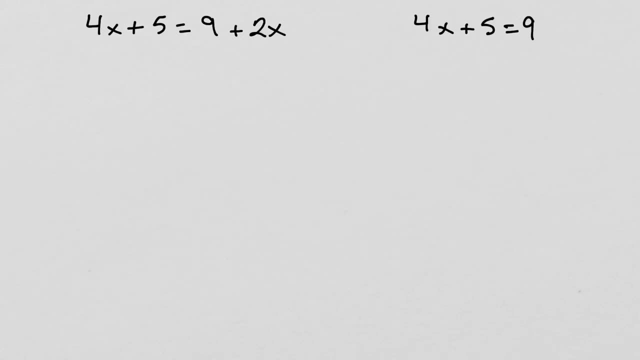 So here you can choose to move the 4x or 2x. I'll move the 2x to the other side of the equation To do that, since the 2x is adding, you will subtract 2x from both sides. 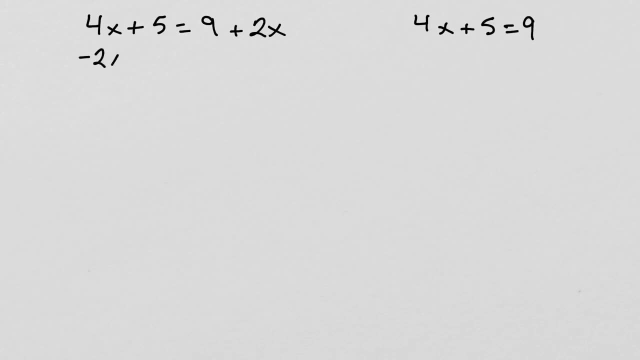 of the equation, The 2x will cancel out. Now, 4x minus 2x is 2x, So we have 2x plus 5 equals 9.. We now have a familiar two-step equation which you should be able to solve if you've. 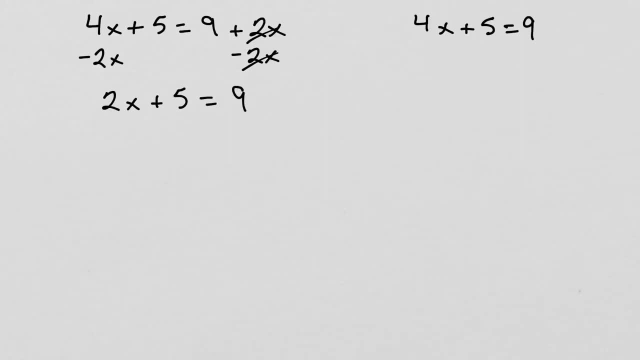 watched our previous videos, But let's go over it. We want to get rid of all the numbers attached to the x so we can have the x alone on one side of the equation. To achieve this, we know that we must get rid of the times 2 and the plus 5.. Let's write: 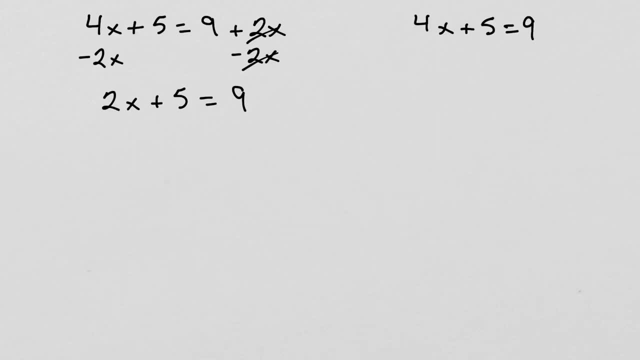 our order of operation. Please, you don't need to be writing the order of operation in your solutions. at school, We are using it for teaching purposes. We are using the reversal of the order of operation, so we are working from the bottom up. 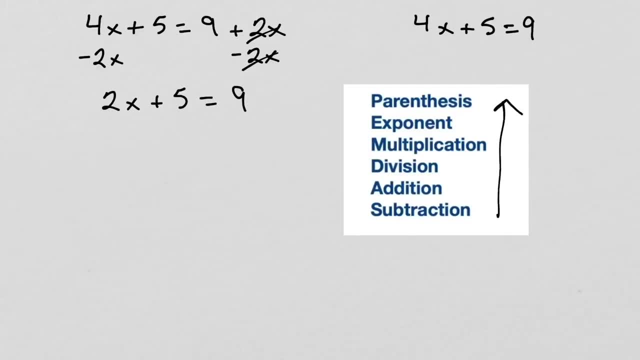 We will see that in this form we must do the addition first and the multiplication second To get rid of the plus 5, we must perform the opposite operation on both sides of the equation, So we will subtract 5 from both sides. 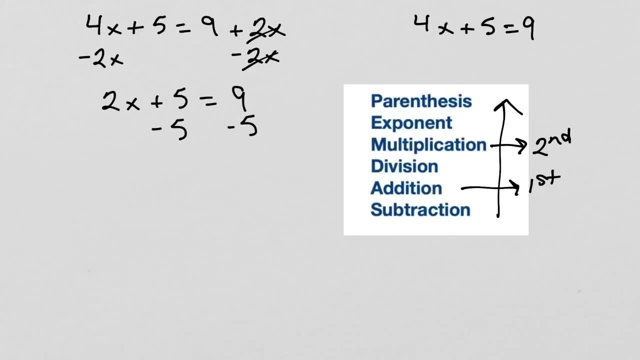 Step 3: Great Step 3 x equals 3 раза, is 3x Step 3.. Next we will divide x by 3. Step 4 x equals 2. Step 3 x equals 4. The 5 cancels out. 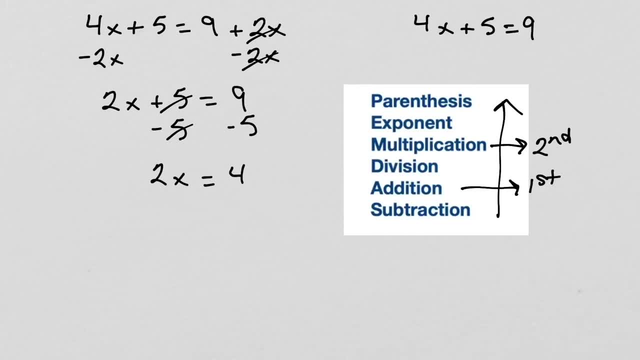 Nine minus five is 4.. We now have 2x equals 4. So we have 2x equal 4.. All right. Next we will get rid of the multiplication by 2. We do this by performing the opposite operation on both sides of the equation. 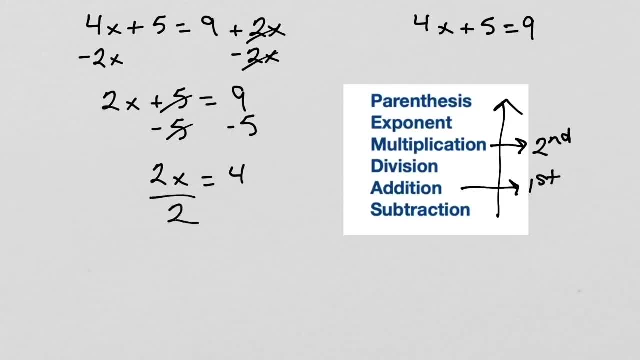 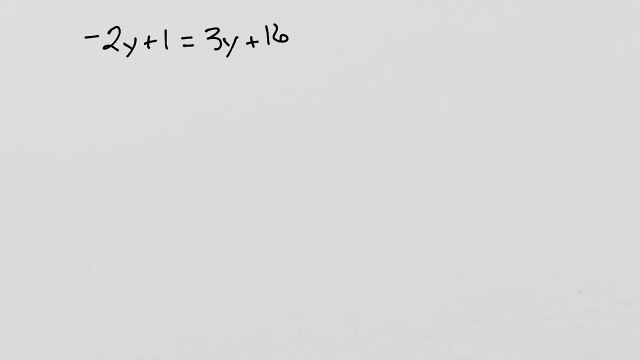 Step 4 x equals 4. Step 4: x equals 4. by 2.. The 2 will cancel out: 4 divided by 2 is 2.. Therefore x equals 2.. Let's take another example: Negative 2y plus 1 equals 3y plus 16.. Solve for y. Here again we want. 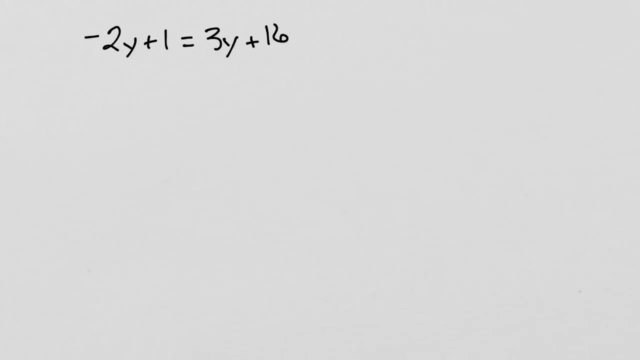 to first move the y's to one side of the equation. You can choose to move the negative 2y or the 3y. I'll move the negative 2y to the other side of the equation To do that, since we 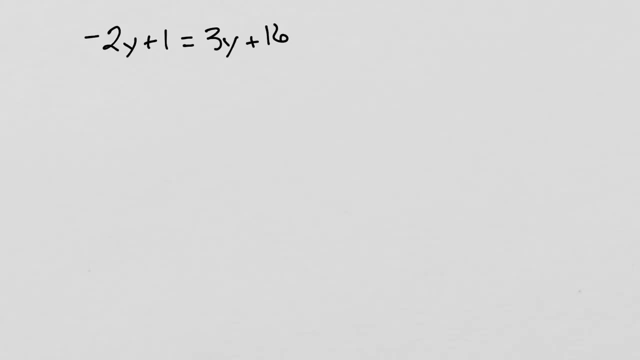 have negative 2y, I will add 2y to both sides of the equation. The 2y will cancel out. Now 3y plus 2y is 5y, So we have 1 equals 5y plus 16.. We now have a familiar. 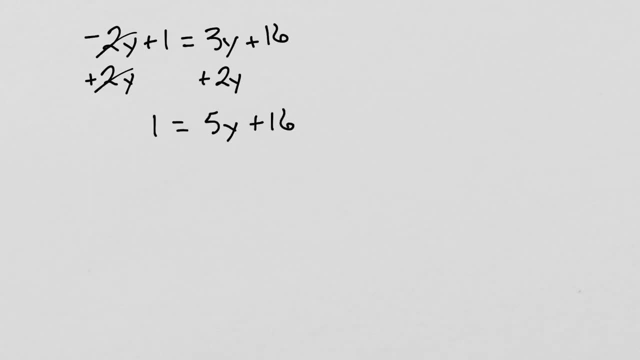 2y equation. Let's take another example. Let's try it again. So we have 1 equals step equation which you should be able to solve, but let's go over it. We want to get rid of all the numbers attached to the y so we can have the y alone on one side of the. 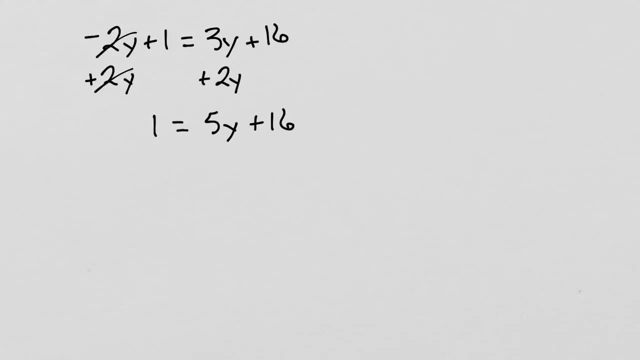 equation. To achieve this, we know that we must get rid of the times 5 and the plus 16.. Let's write our order of operation. We are using the reversal of the order of operation, so we are working from the bottom up. We will see that in this form we must do the addition first and the multiplication. 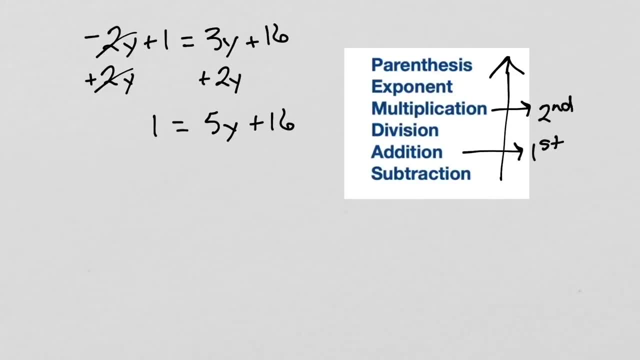 second, To get rid of the plus 16, we must perform the opposite operation on both sides of the equations. So we will subtract 16 from both sides. Subtitles by the Amaraorg community. The 16 will cancel out. 1 minus 16 is negative 15.. 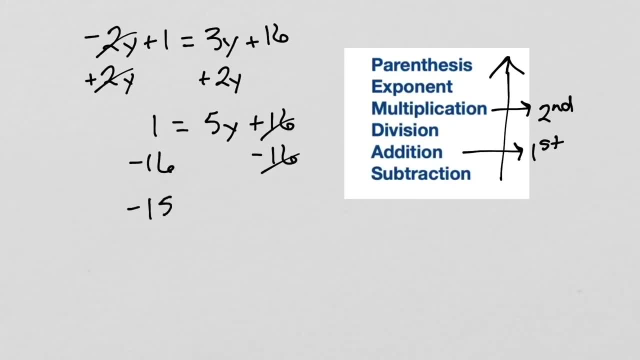 We now have: negative 15 equals 5y. Next, we will get rid of the multiplication by 5.. We do this by performing the opposite operation on both sides of the equation, So we will divide both sides by 5. The 5 will cancel out. Negative 15 divided by 5 is negative 3.. Therefore y equals negative. 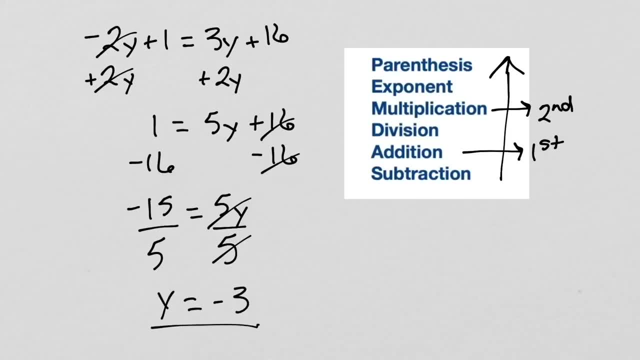 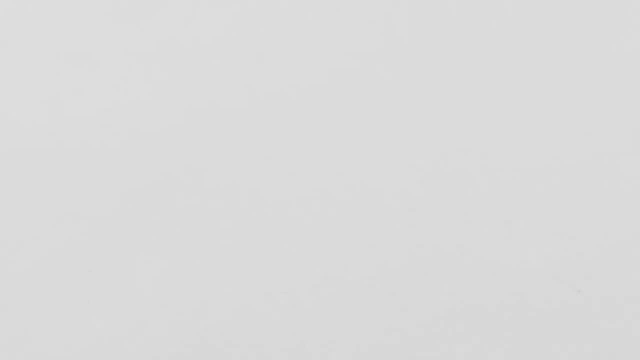 3. Subtitles by the Amaraorg community. Let's look at a more complex example. Some equations require initial operations to simplify them before you can even start to solve them. 2x minus 4 equals 5 parentheses x plus 1 parentheses minus 4x. Solve for x When you have a question. 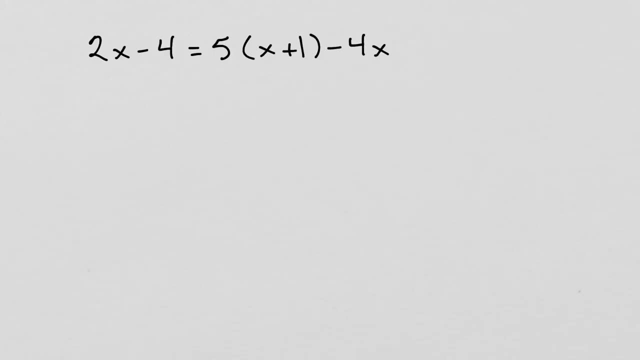 like this: your first step is to distribute the 5. So that you can have the x out of the parentheses. So the 5 will multiply the x to get 5x, And the 5 will multiply the 1 to get 5.. 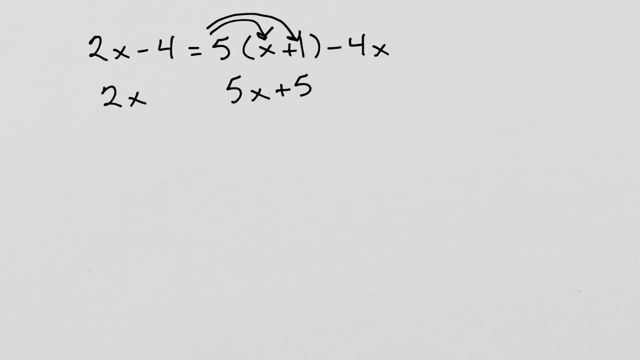 So now we have 2x minus 4 equals 5x plus 5 minus 4x. Subtitles by the Amaraorg community. Subtitles by the Amaraorg community. Subtitles by the Amaraorg community. Next we can work on the 5x minus 4x to get 1x. 1x is the same as simply x.